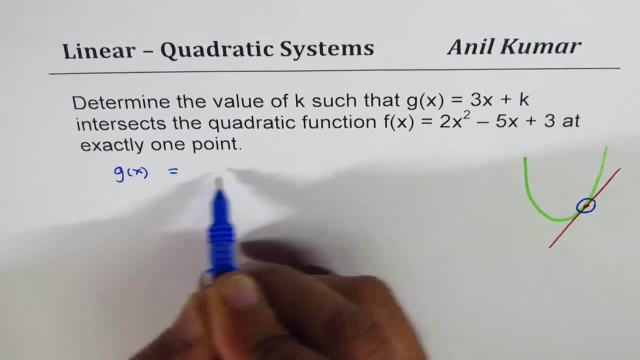 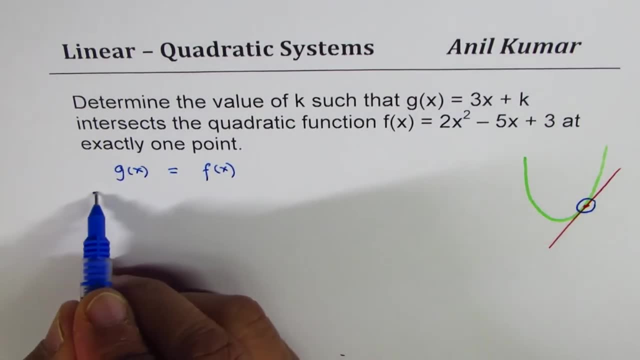 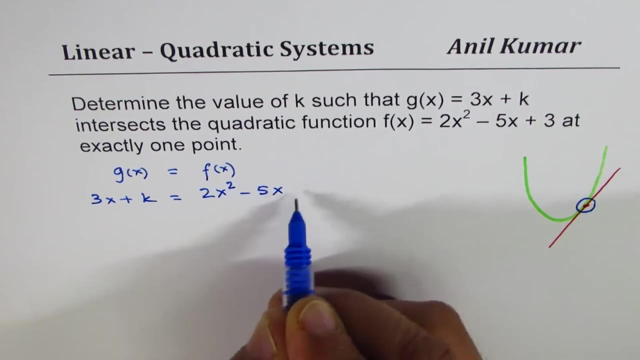 should be same, So g of x should be equal to f of x, right? So you understand why I've written this. Now. g of x is given to us as 3x plus k, and f of x is 2x square minus 5x plus 3.. 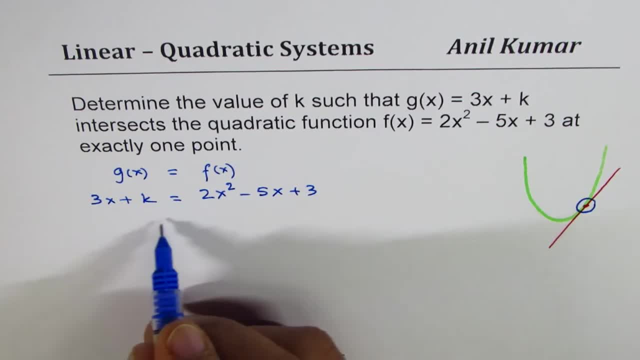 They should be equal, So let's bring them to one side. solve for x, right? Okay? So we get here 2x square minus 3x. We already have minus 5x plus 3 minus k. Okay, Combine the like terms, So we get 2x square. 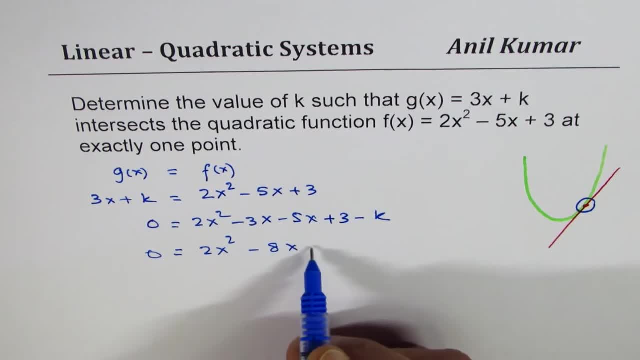 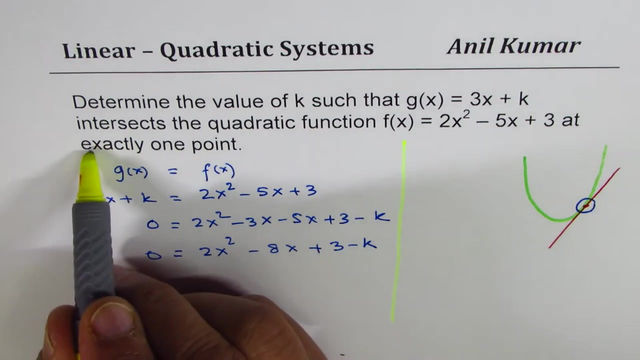 minus 8x plus 3 minus k, So that becomes a quadratic equation. basically, Now, a quadratic equation could have one solution, two solution or no solution. right Now, what is the condition for this equation to have One solution? Since we need exactly one point, we need one solution, right. 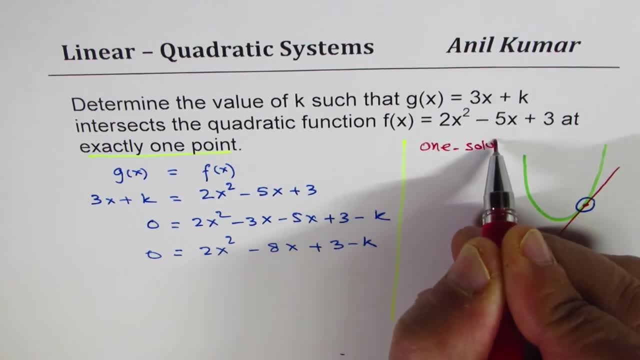 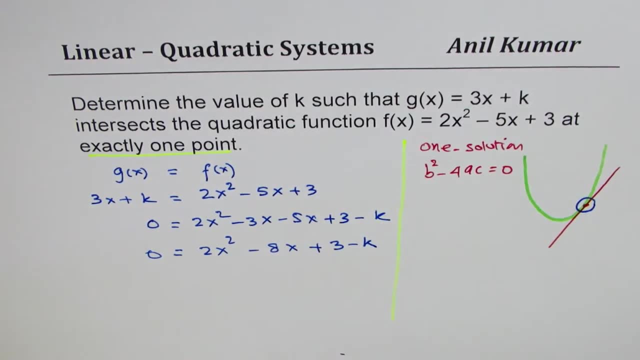 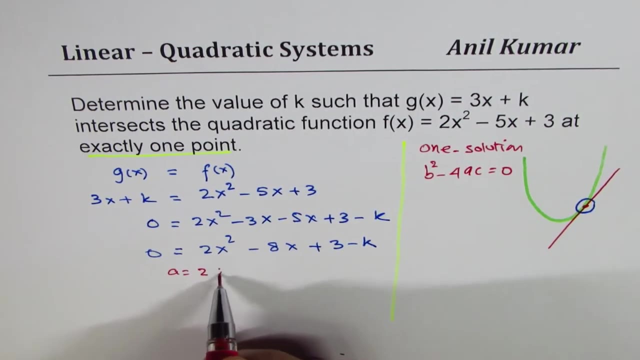 So for one solution the condition is: b square minus 4ac is equal to 0, right, That is what the condition is Now in our equation. what is a, what is b and c? So here a is equal to 2,, b is equal to minus 8, and what is c, c is? 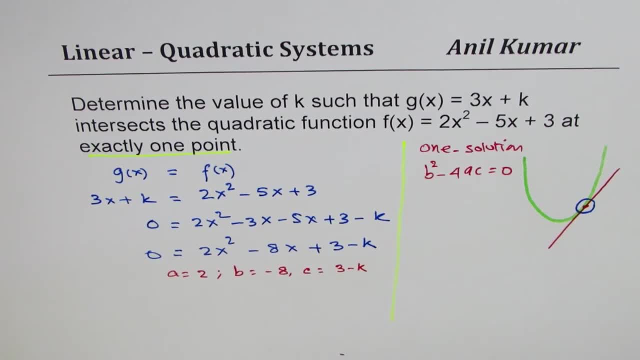 3 minus k, the constant correct now i hope you can do it very easily. so basically we'll replace all these numbers and find k, equating it to 0. right? so b square b is minus 8. so we'll do minus 8. square minus 4 times a is 2 and c is 3 minus k. so at this stage what we have done is 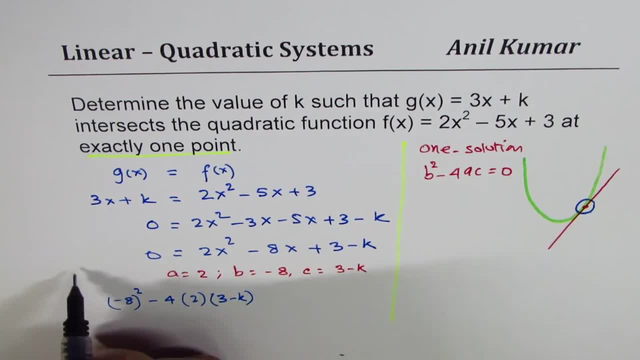 we are equating b square minus 4ac to 0. where a is 2, b is minus 8, c. is this right? so we are equating this to 0. that's the whole idea and that helps to solve. correct. so we get 64.